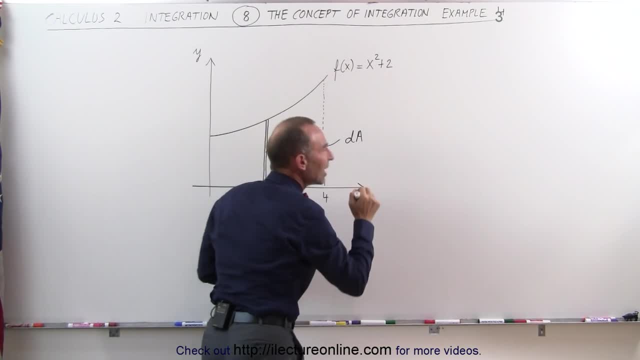 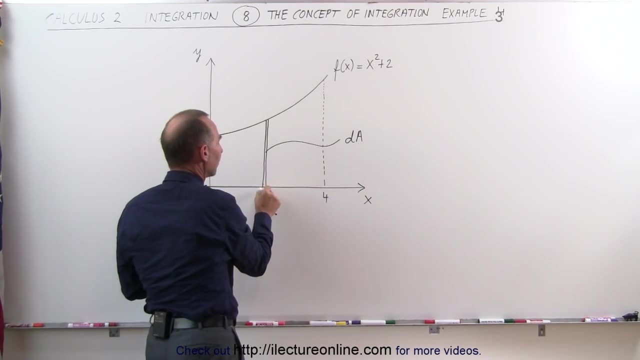 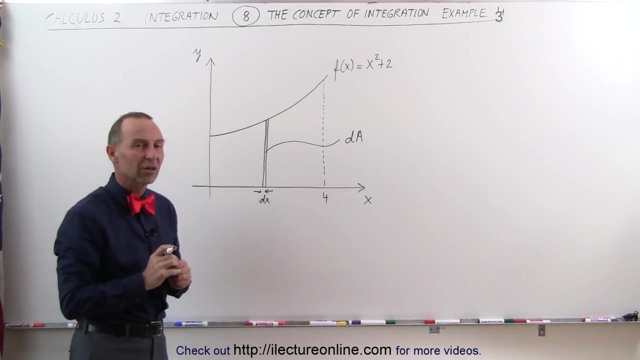 that small amount of area, a dA, like a small change in area, a very small, minuscule amount of area. That area is equal to the height of the rectangle times the width of the rectangle, and the width of the rectangle is going to be a very small amount of dx, a very small change in x, a puny, tiny, tiny. 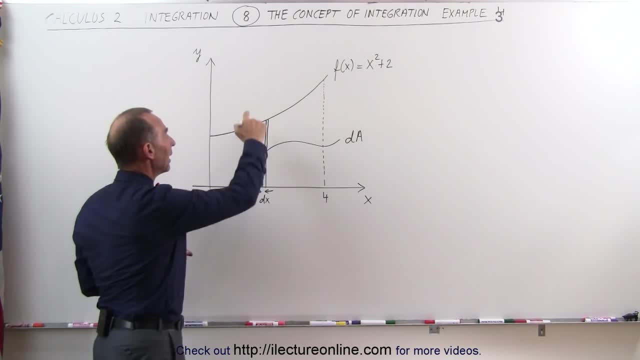 little change. So that's a very narrow little rectangle and the height will be the function evaluated at this particular value for x. So whatever this value for x is, I plug that value into my function and I evaluate it. I get an f of x and that will be the height of the rectangle. 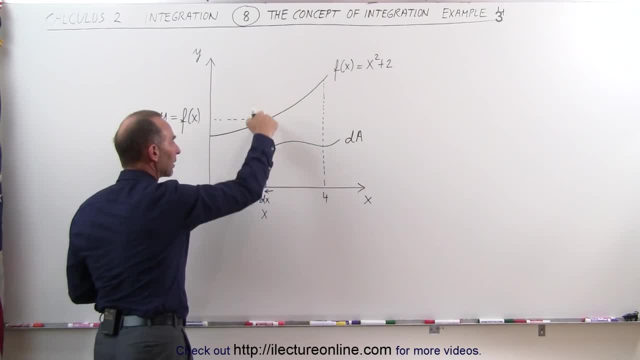 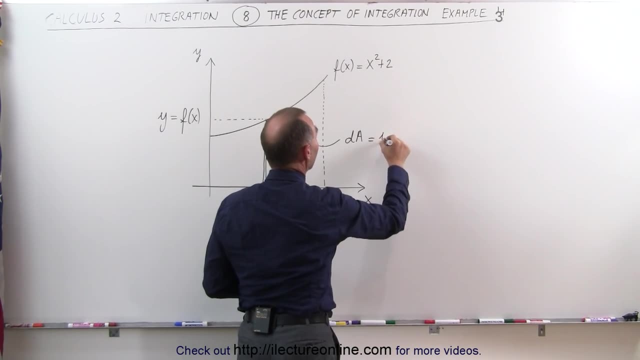 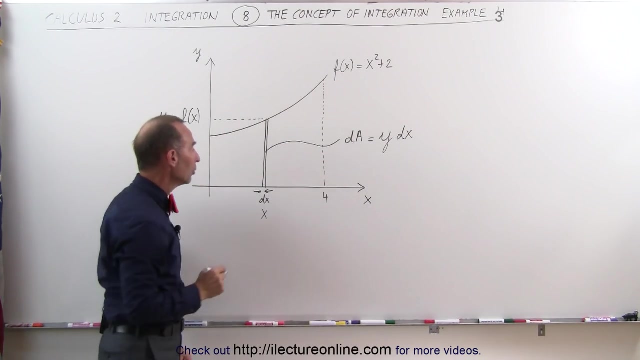 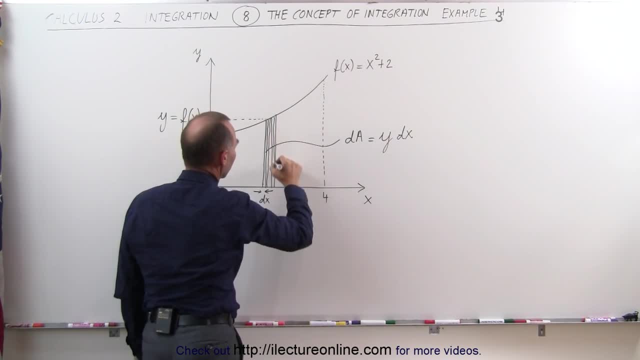 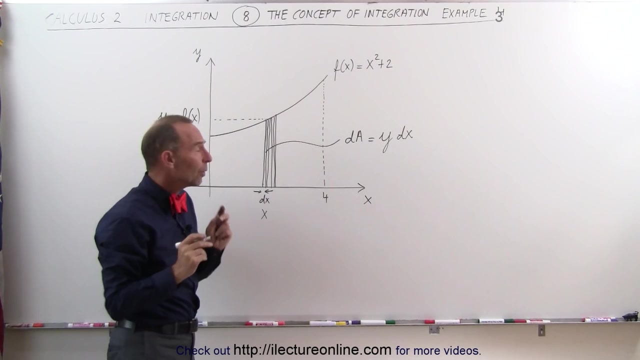 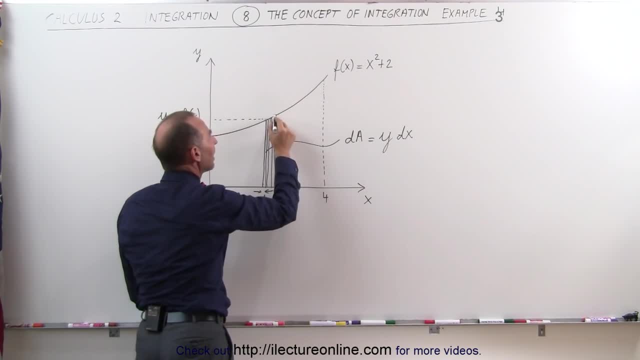 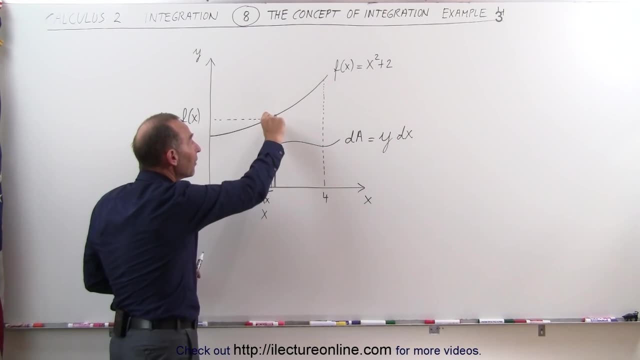 minute. if you come up here and you look at that, you can see that the area of each rectangle is not exactly equal to the area underneath the curve. at that particular location You have a little bit of excess area and remember that. to solve that problem, we just need to make the width of each. 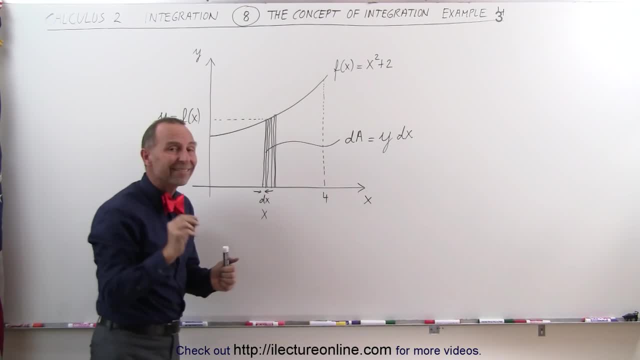 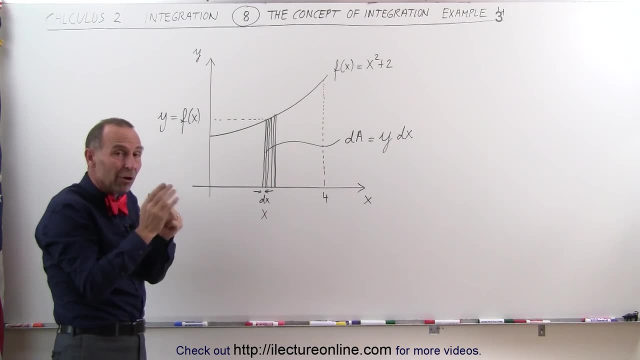 rectangle a little thinner. we make the rectangles the less area you have sticking out there in that one corner and in the limit. if we just make the thickness of the of the rectangles thin enough, where delta x goes to zero, where the thickness goes to zero, then eventually, if i add up an infinite number of rectangles, 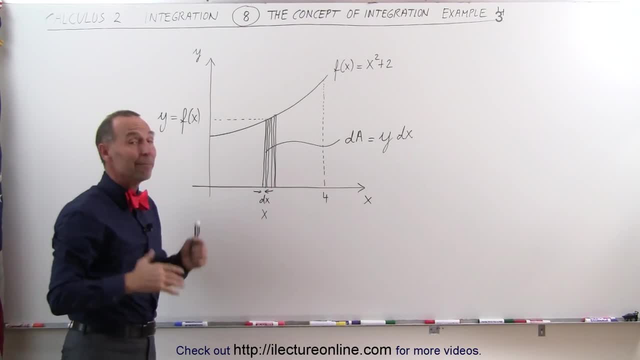 that should add up to exactly equal to the area you need to curve and, by definition, the integral of the function of x times dx. evaluated from the lower limit, let's say from zero all the way up to the upper limit, four equals the area underneath the curve. in other words, when we go to the limit. 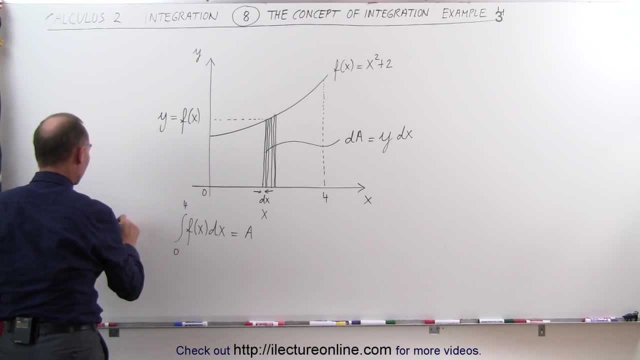 when delta x goes zero, that is equal to this. so this is equal. the area is equal to the sum of all the areas, of all the little rectangles, from i equals one to infinity. when we do that- and of course we can't say that it's equal to infinity- the area is equal to the limit. 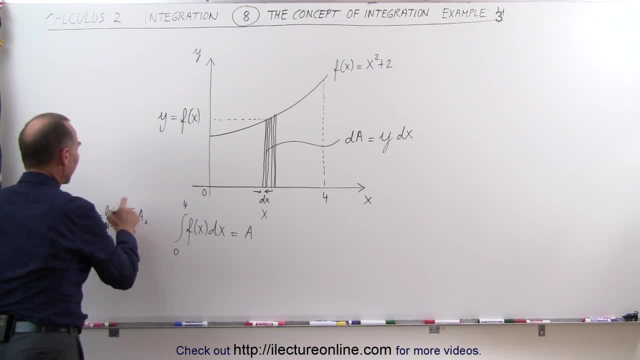 as n goes to infinity and if we replace that by n, So if I have n number of rectangles and there's almost an infinite number of them, if n approaches infinity, all those sums of all those rectangles added together will add up to the exact area I need to curve. 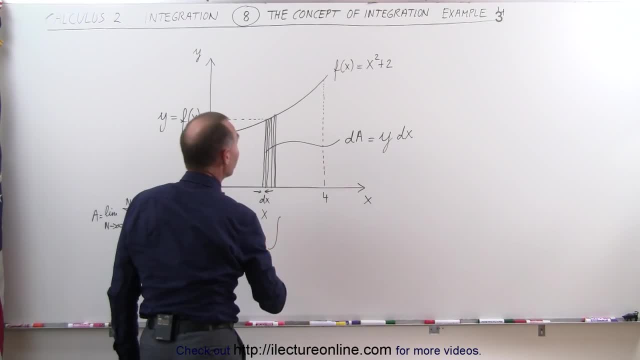 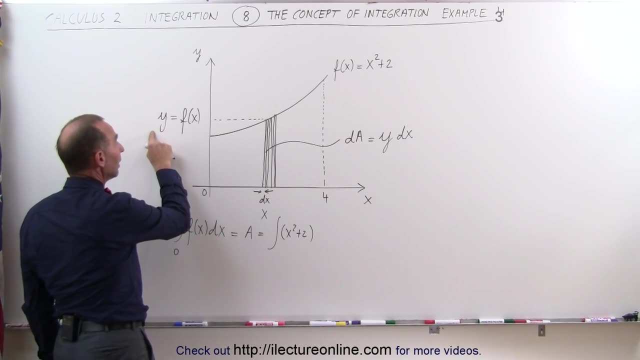 And so to find the exact area of the curve, this is equal to the integral of the function, which is x squared plus 2.. Remember that the function which is equal to y is indeed, in this case, x squared plus 2,. 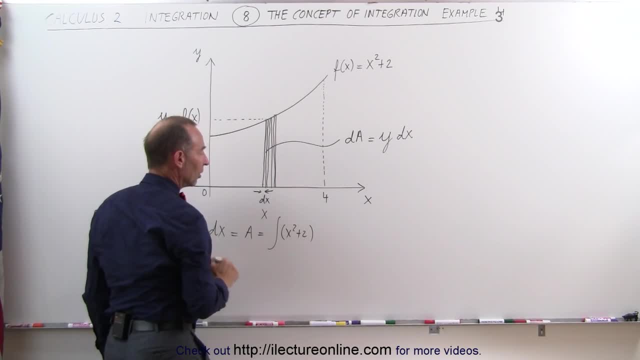 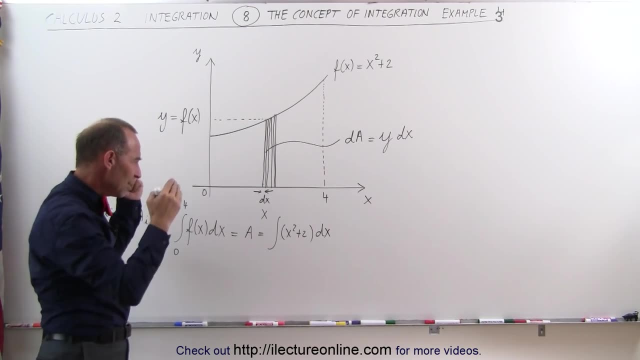 so that's the height of each rectangle at each value for x. We multiply that times the dx, which is the width of each rectangle, and that's where that dx came from. If you always wondered, why does he keep putting a dx there? 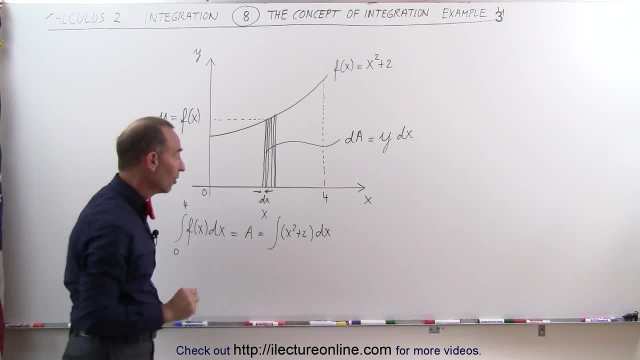 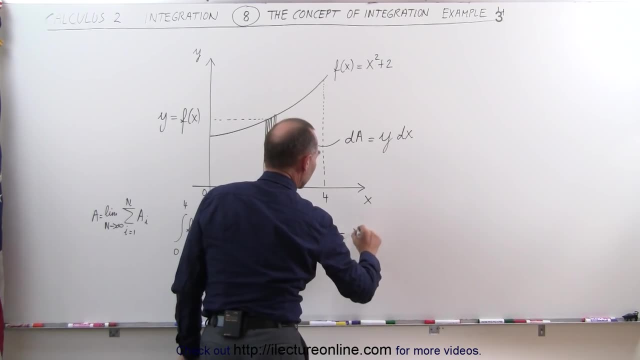 it's because it represents the width of each of the rectangles. We evaluate it from x equals 0 to x equals 4, and then if we integrate that, we get x cubed over 3 plus 2 times x. Remember you always add 1 to the exponent. divide by the new exponent. 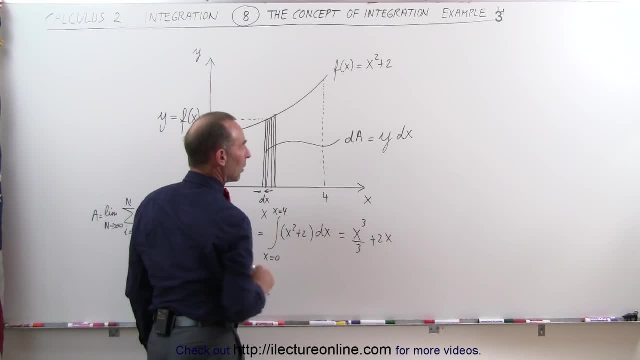 Here we have 2x to the 0, that becomes 2x to the 1 divided by 1.. And then we evaluate that from the lower limit to the upper limit. It means we plug in the upper value. This is equal to 4 cubed divided by 3 plus 2 times 4.. 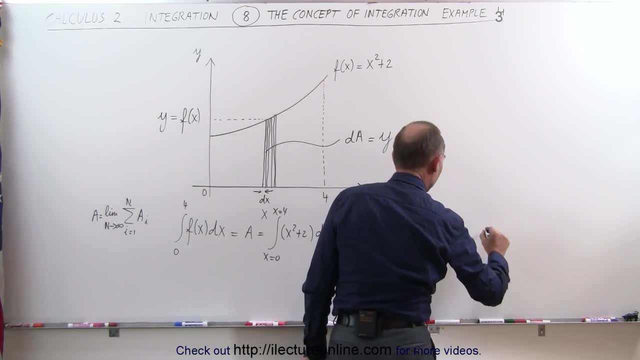 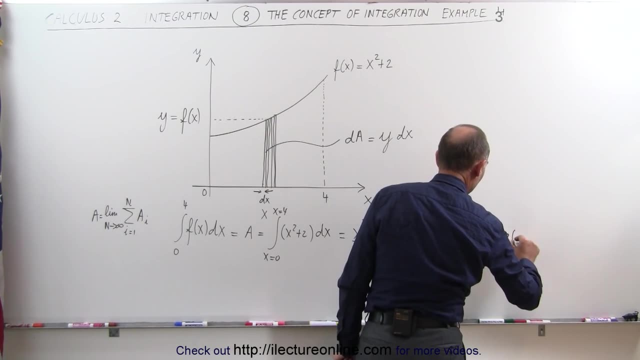 So we replace x by the upper limit and then we subtract from that When we plug in the lower limit, which is 0 cubed divided by 3 plus 2 times 0.. Of course we didn't need to do that because we could see that when we plug in 0 for lower limit. 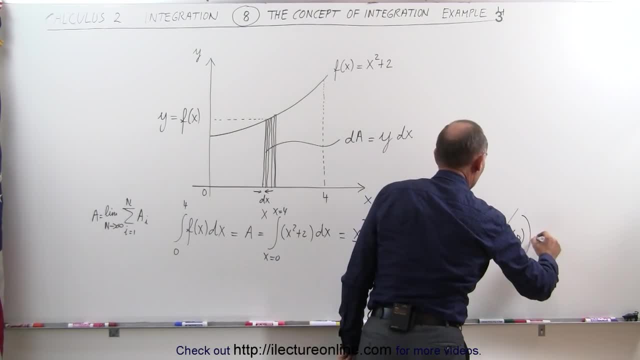 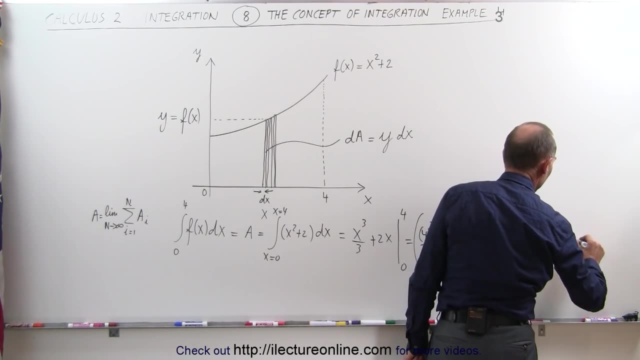 it just goes to 0. So this simply disappears and that is equal to 64 divided by 3 plus 8.. 64 divided by 3 is equal to 21 and a third plus 8. So eventually we could say that's 29 and a third is the total area underneath that curve.